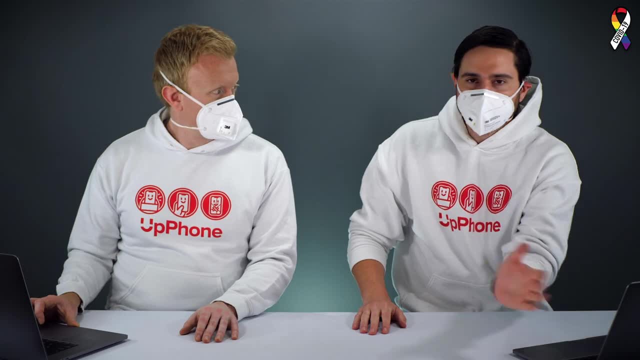 Yeah, We went from 231 to 144.. We already knocked out 90 plans that you didn't need. Yeah, I like it. Let's say we want to do a two-line plan, So now we're down to 75 plans. 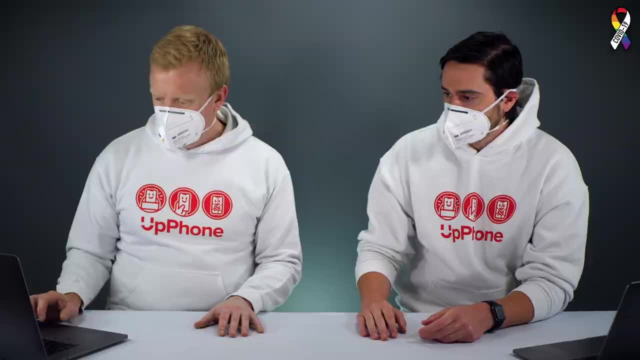 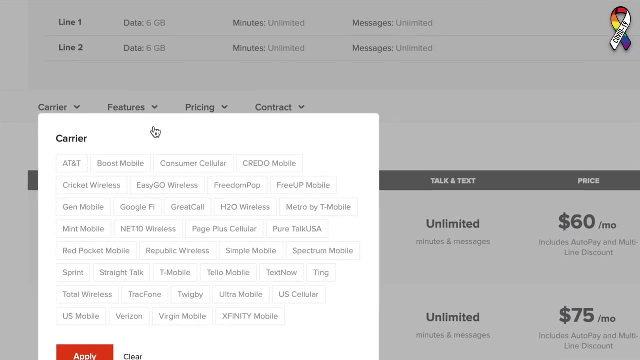 We've now cut it in half again, So we're really narrowing this down And you have some other menus you can use to filter the plans. You can sort by carrier. If it's a specific carrier you have in mind, check that out. 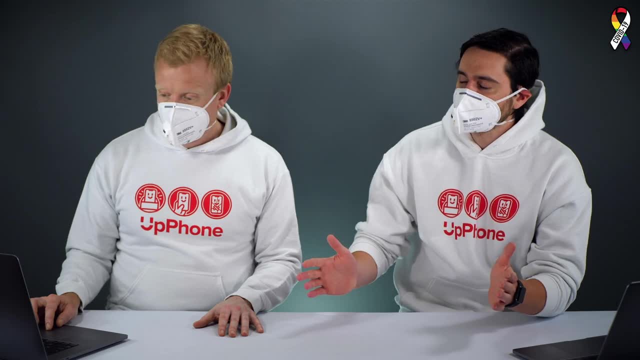 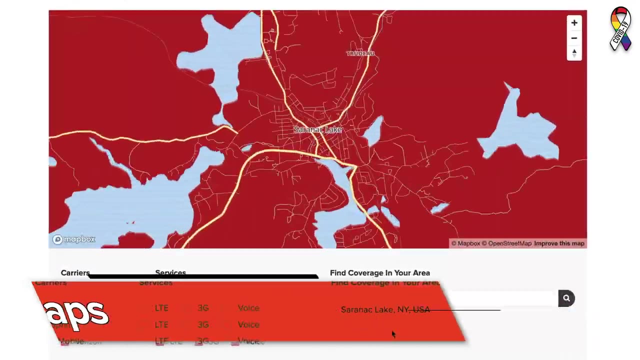 But before you choose a carrier, if you have one that you're set on, check wireless coverage too. The worst thing you can do is switch to a carrier that doesn't have coverage where you live. Yeah, So check out upphonecom slash maps. 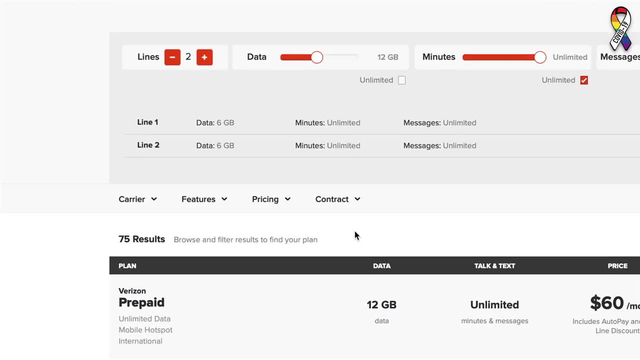 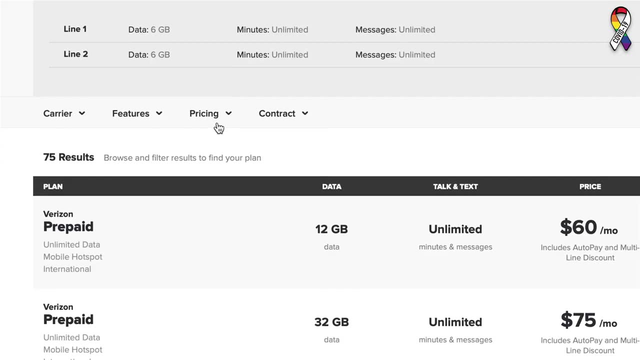 and you'll find our coverage maps there. So the next menu. there is features. Maybe you want mobile hotspot, Maybe you want unlimited data, Maybe you want international calling. You can select that there. Pricing: What's your desired price range for a plan? 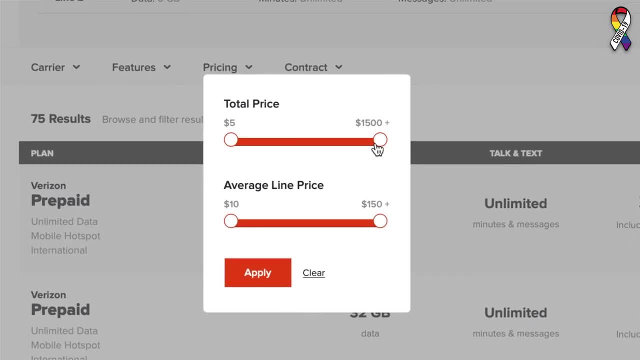 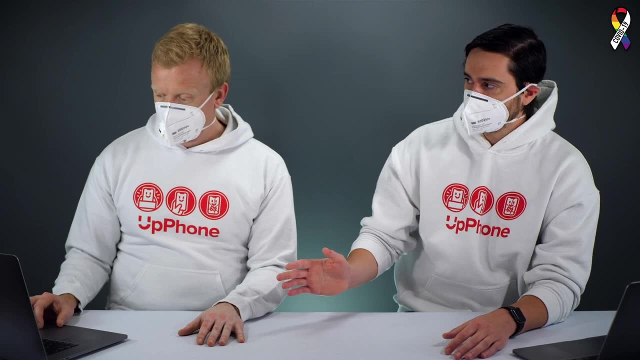 Really, these days you can get plans for as little as $10.. You can get an unlimited plan for as much as $100 a month. So really it's up to you what you're comfortable paying. You don't have to pay a lot of money for a great cell phone plan. 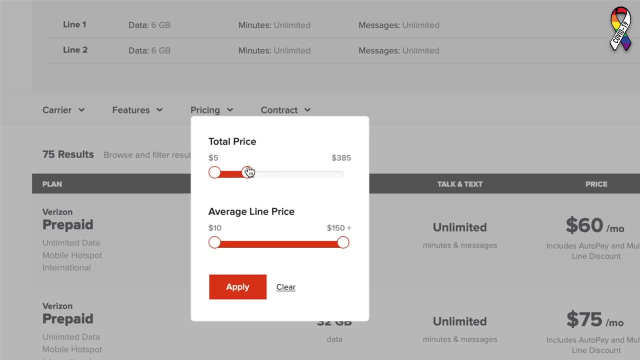 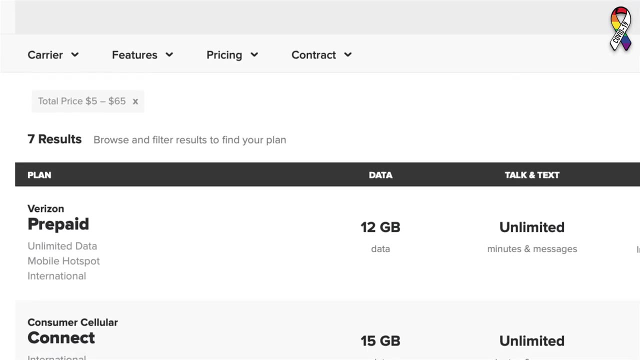 That's one of the things we like to talk about a lot. So for our two-line plans, let's filter. Let's say we want to pay a maximum of $65.. All right Down to seven results. We're really narrowing this down. 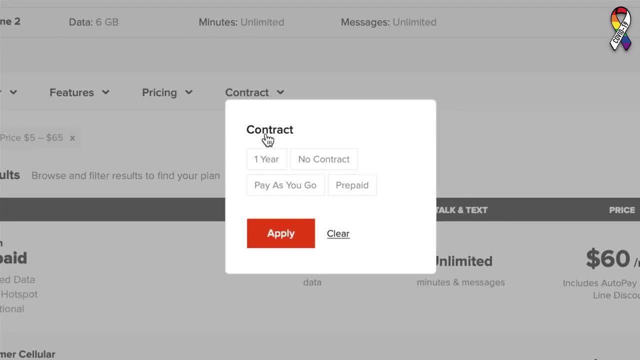 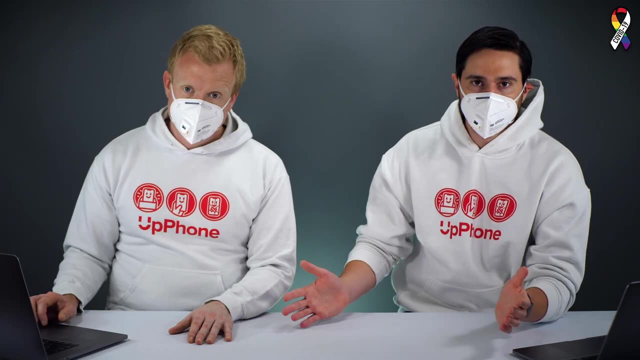 And then the last column. there is contract Prepaid, No contract Pay-as-you-go. We like to give you all of your options. even though we personally don't recommend pay-as-you-go plans, They are a good fit for some people if you don't use your cell phone a lot. 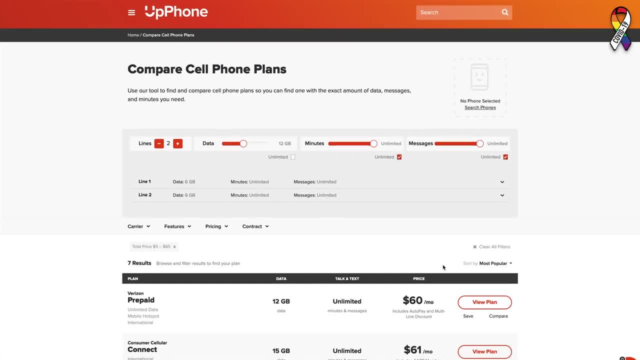 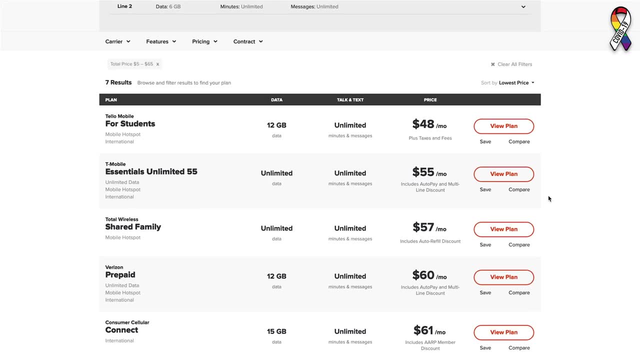 So that's why that's there. We've narrowed it down to seven plans. Let's take a look at some of these And we can sort too. Let's sort by the lowest price. So, as you can see there, the cheapest plan that falls under our criteria is from Telomobile. 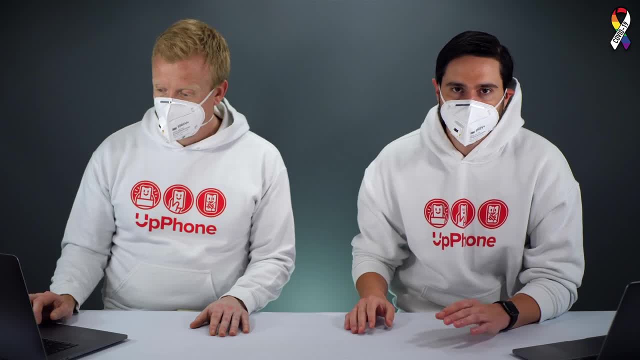 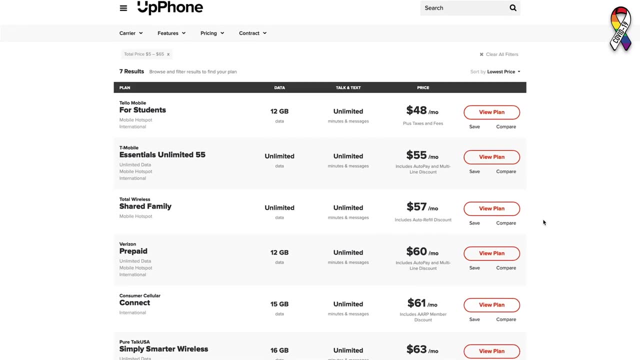 Great carrier. They are a Sprint mobile virtual network operator that leads coverage from Sprint. I just think that we should take a look at that Verizon prepaid plan. This is our favorite plan. We didn't actually design the video to do this way, but the Verizon prepaid plan is our favorite plan. 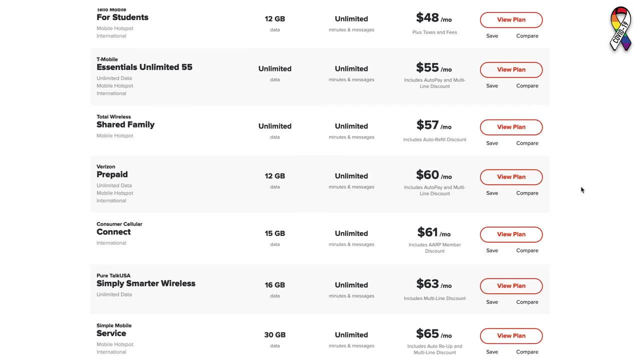 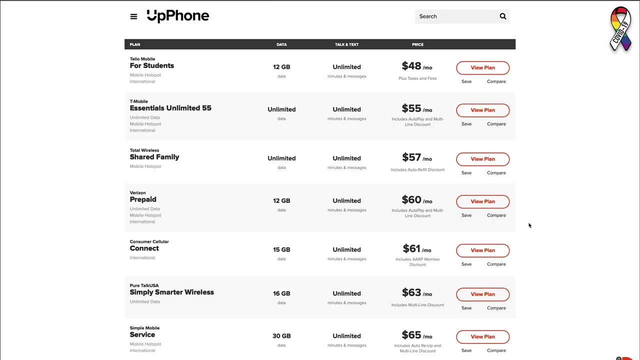 And it's cool that it actually worked out that our dummy person found this plan above. Come on, David. Well, let's say they can also compare the plans too. Yes, So if you wanted to, for instance, take a look at Verizon's prepaid plan. 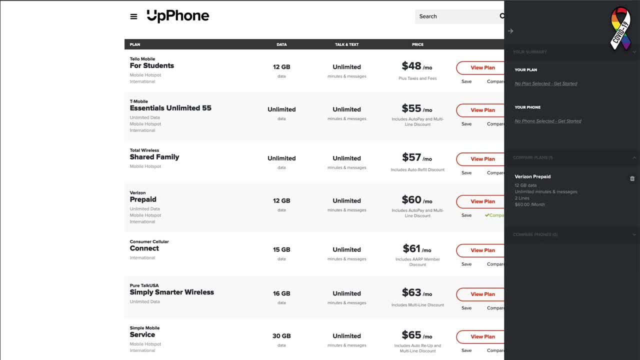 We've got our little drawer over here. This is going to help you to compare, And let's say the PureTalk plan and then the shared family plan by Total Wireless, And then over here you can just click full comparison. This will bring you to a page where you can just compare everything side by side. 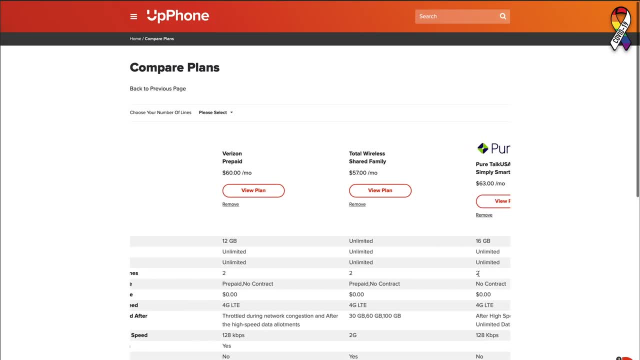 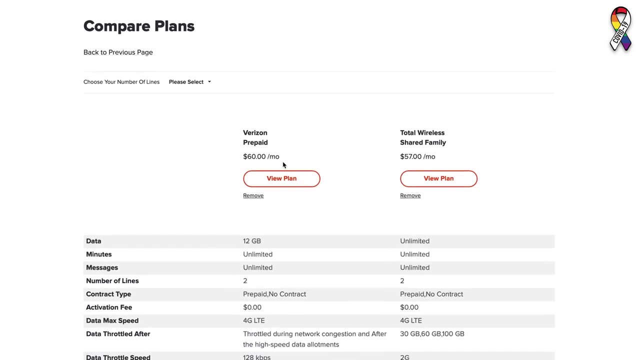 Scroll back and forth. Got PureTalk Verizon prepaid And you can see the contract types and the amount of data, minutes and messages and other things, And then you can view more information about that plan by clicking view plan. Yeah, let's go ahead and do that. 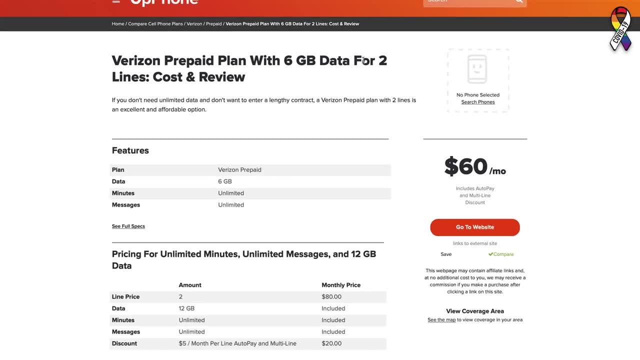 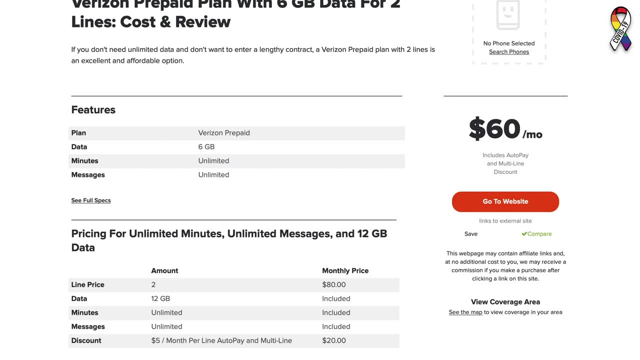 So this is going to bring us to Verizon prepaid plan with six gigabytes of data for two lines. So it's going to give us a total of 12 gigabytes of data. We see that down here. Super easy synopsis right at the top. 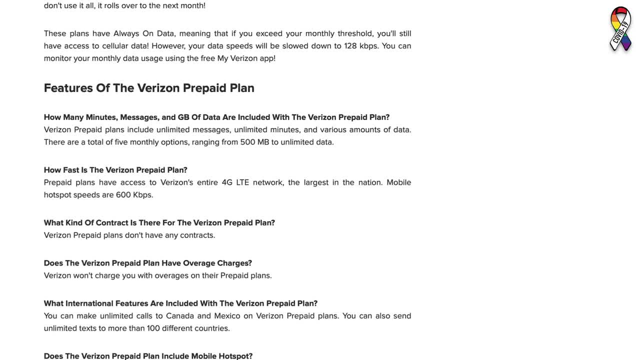 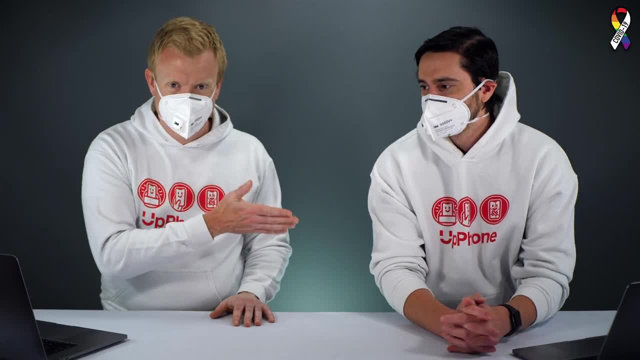 We just wanted to put all the information there for you to see. Next, we have details about the plan And we personally went and reviewed every single plan. David, Yeah, Wrote a lot of that Is the man for all this stuff. 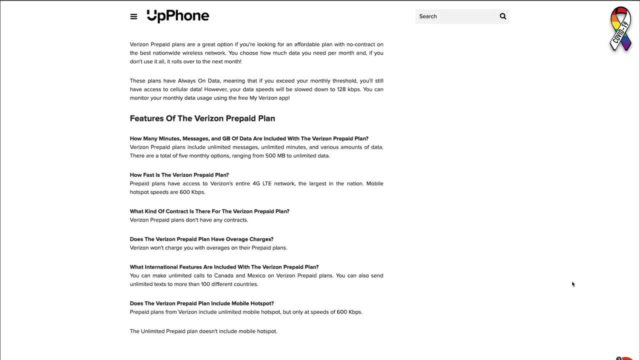 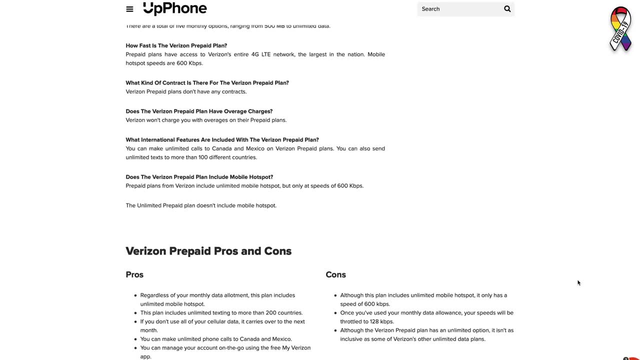 He's the man with the plans. Yes, So let's talk about minutes, messages, data, how fast the plans are? mobile hotspot: Does it have international calling features? There's a lot of stuff here. Yep, Yep. Pros and cons of the plan. 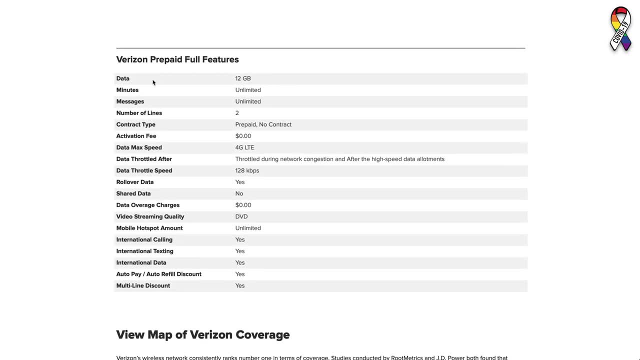 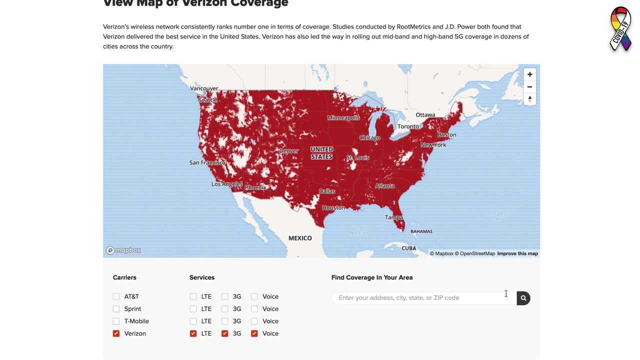 You can also view some other Verizon prepaid plans there. Full feature table down here And then a view map of a Verizon coverage. Yeah, So if you don't know which, if you're shopping around, not sure if the carrier has coverage where you live. 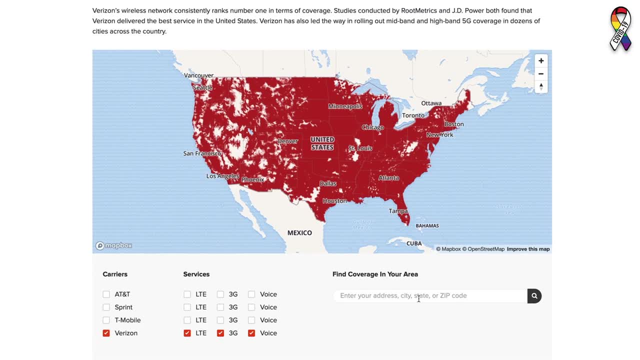 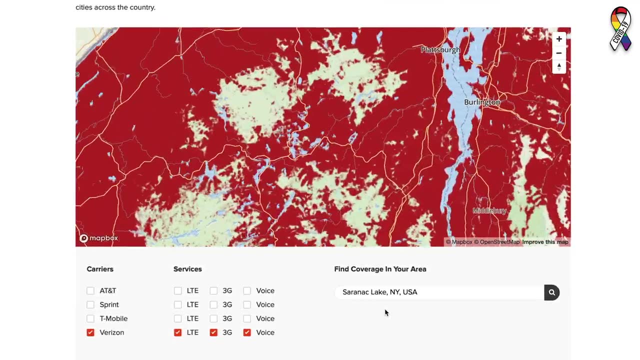 you can check right on the page of the plan. Yeah, So if I wanted to see what coverage was like in, say, Saranac Lake, New York, just type that in. You can type in your exact address too, And Apple zoom in. Pretty good. Yeah, Verizon does have coverage in Saranac Lake. Yeah, I actually had to switch. I was on Virgin Mobile. They were also a Sprint mobile virtual network operator. My service wasn't so good. Switched to Verizon. 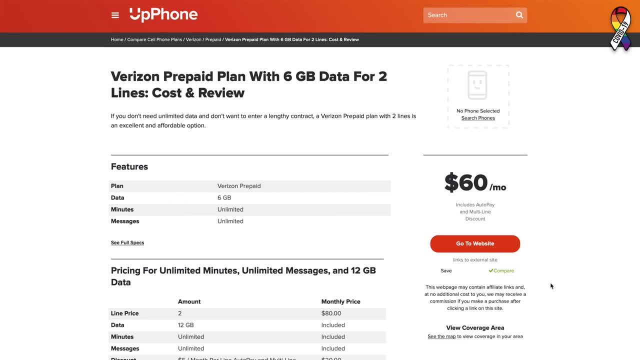 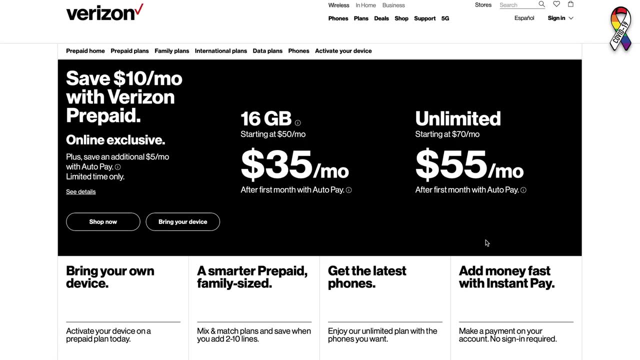 It got much better. When you found a plan that you love, just click the big go to website button And it'll shoot you off to Verizoncom. Go through the process, Check out. It should be as easy to compare cell phone plans as it is to compare hotels online. 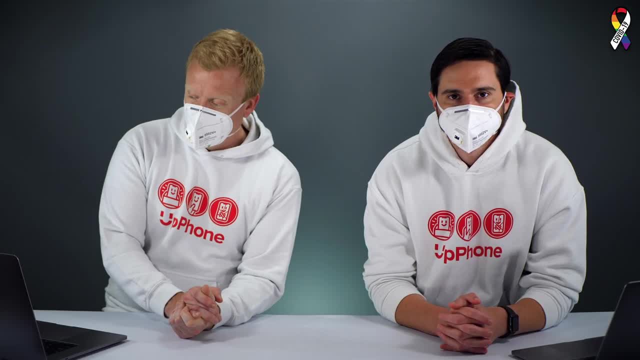 And that was our goal when we designed this website, So we hope that you really enjoy it. We know you will. Yep. Thanks for watching this video. That's how to compare cell phone plans. Give it a thumbs up if you enjoyed.